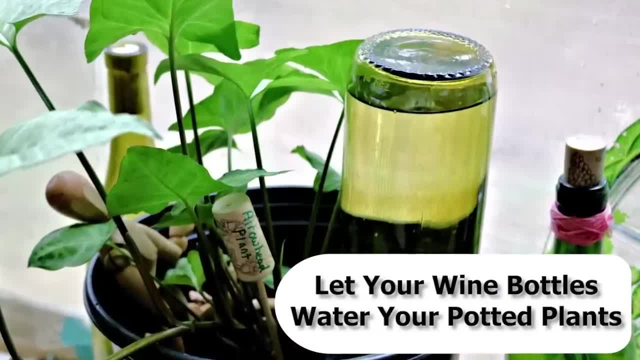 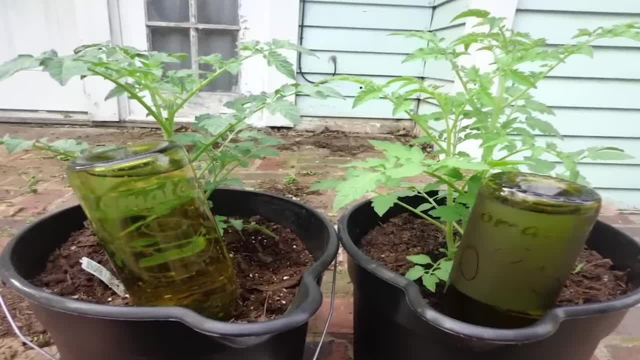 sunflower. Let your wine bottles water your potted plants. One of the biggest mistakes people make with their potted plants is forgetting to water them. If you frequently forget to water the plants or don't have time, you can solve the problem using an empty wine bottle When you've finished. 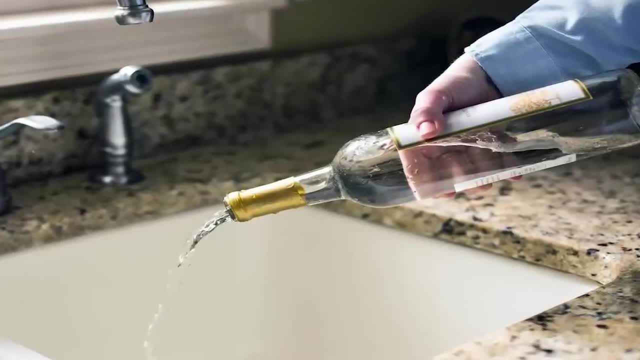 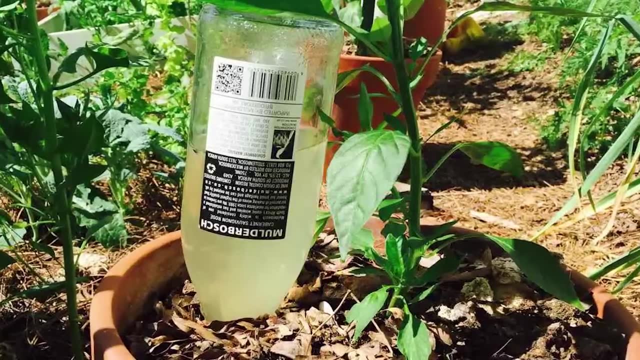 the bottle, rinse it with hot water and fill it with cold water when it's clean. Next, poke a hole in the cork and force it back into the wine bottle. Finally, put the neck of the bottle into the soil and the plant will stay hydrated as long as there's water in the bottle. 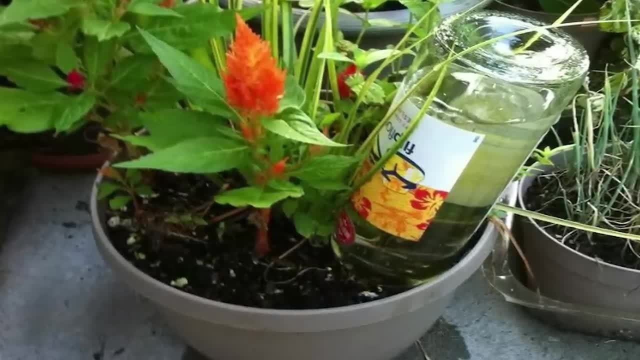 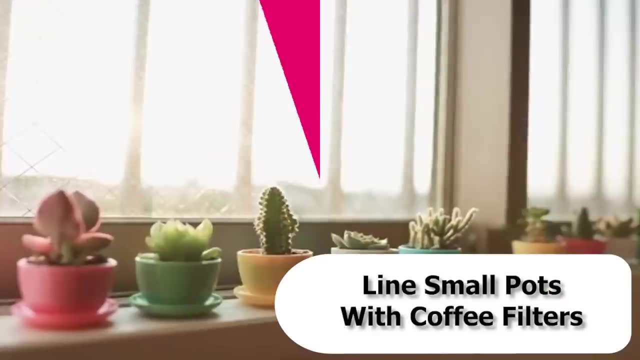 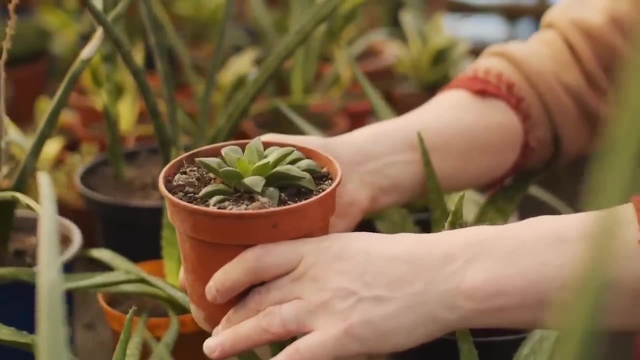 When the wine bottle is empty, refill it with water, put it back in the plant and you'll never have to worry about forgetting to water your plants ever again. Line small pots with coffee filters. Does the water drain from your potted plants as soon as you water them? If so, you know. 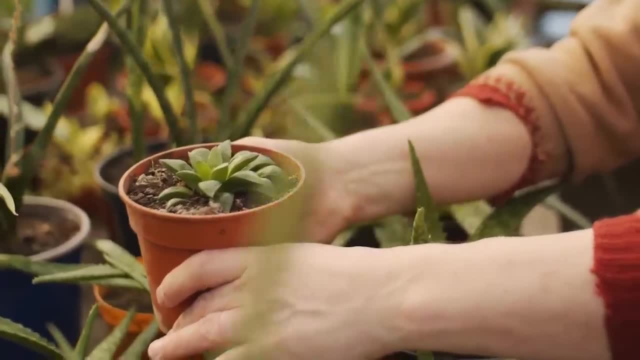 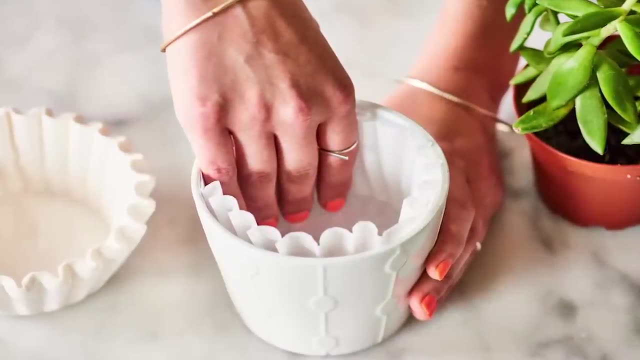 how annoying it can be, since you're probably going to have to do the same to your potted plants. plants need water to thrive. You can slow the leaking process if you have coffee filters in the house. Simply line the bottom of the pots before filling them with soil, and the plant 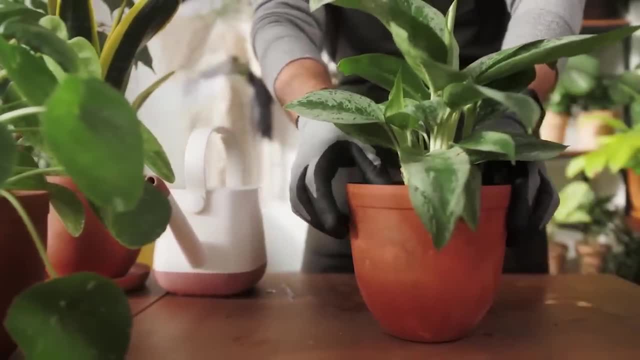 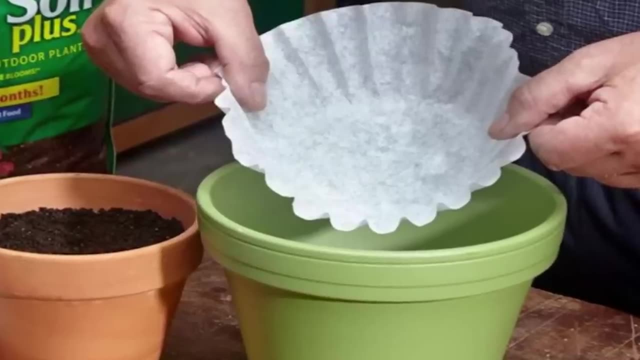 This won't prevent the water from draining, but it will slow things down to allow the soil to absorb the water longer, ensuring it remains moist. Also, lining the pot with a coffee filter will prevent soil from clogging the drainage holes. Keep the deer away. If deer find your 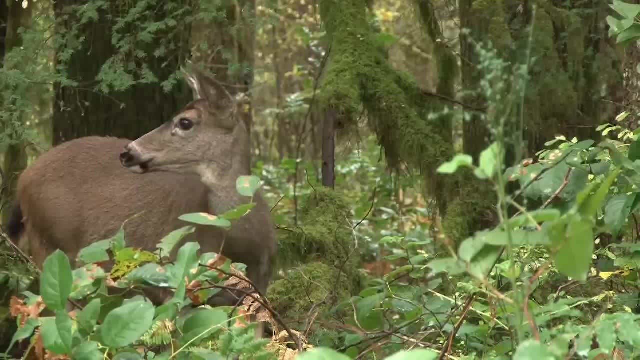 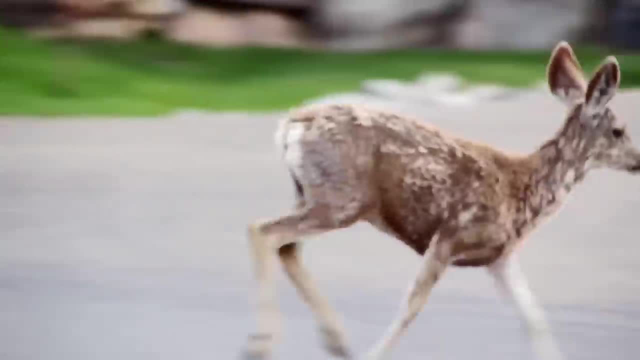 garden. they will wreak havoc and eat the plants and vegetables before you have a chance to harvest. Fortunately, you can solve the problem using a bar of soap. Deer don't like the smell of soap, and placing pieces all over your garden will deter the deer and other critters that may. 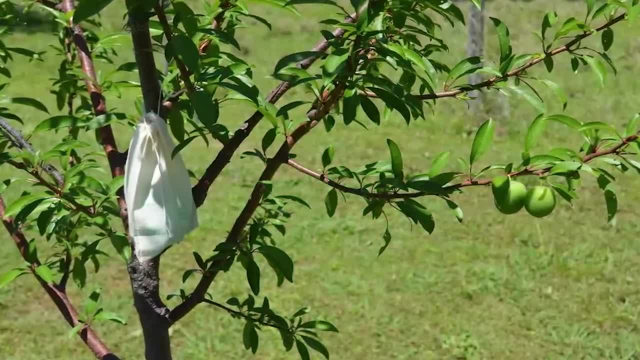 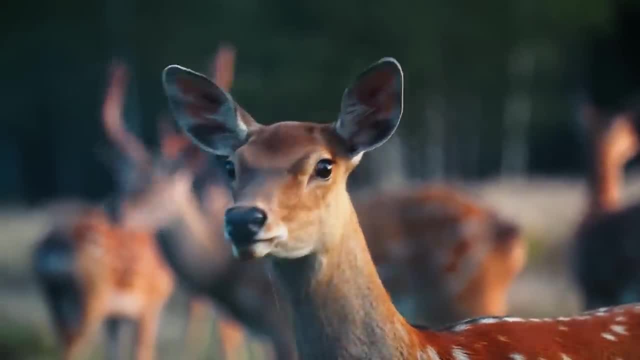 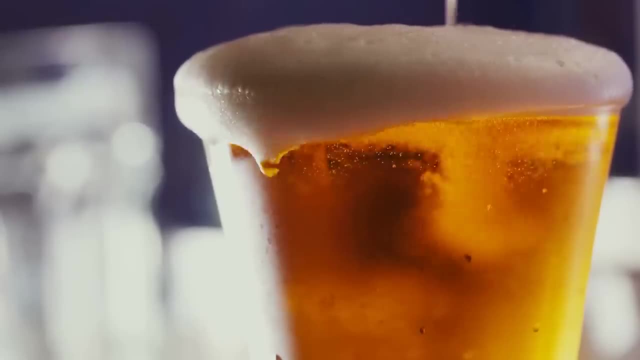 eat your plants. You can also hang the soap from trees around the garden to keep the animals away. It's best to use a highly fragrant bar of soap, because it will be more effective, Another way to deter slugs and snails. Beer is another option if you don't want your garden littered with eggshells to keep the snails. 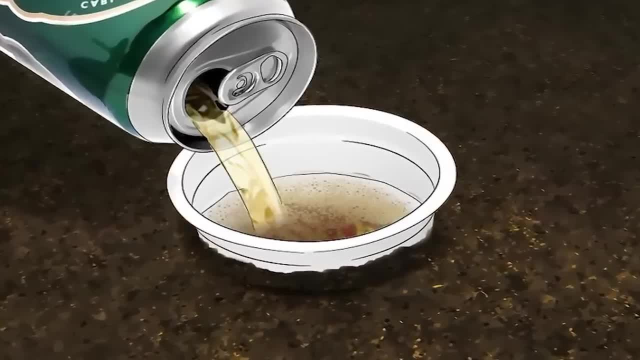 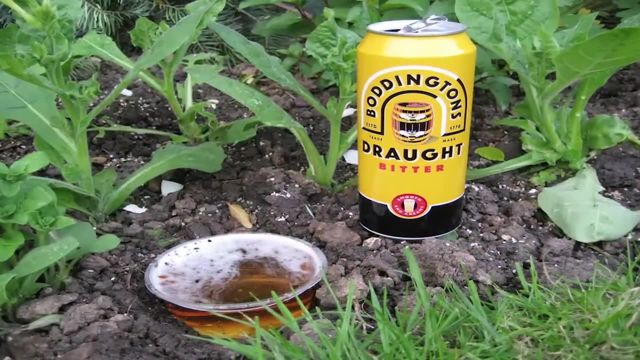 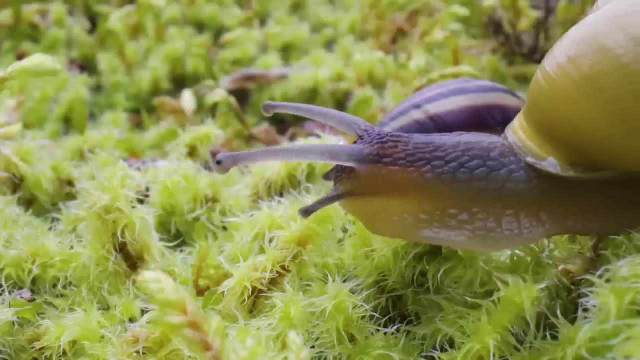 and slugs away. These pests love beer because of the yeast, and you can use it to keep slugs and snails out of your garden. You can fill a tin can with beer and dig it into the ground, away from your plants, and the slugs and snails will gravitate to the can because these pets prefer. 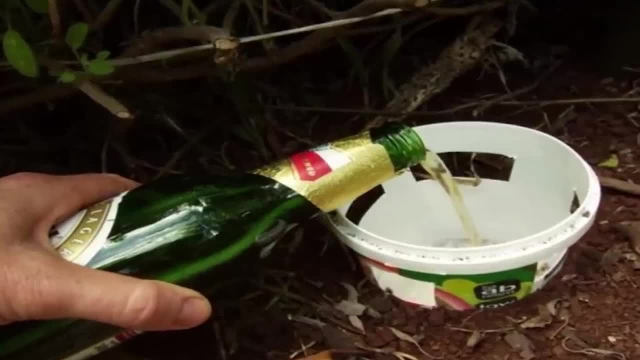 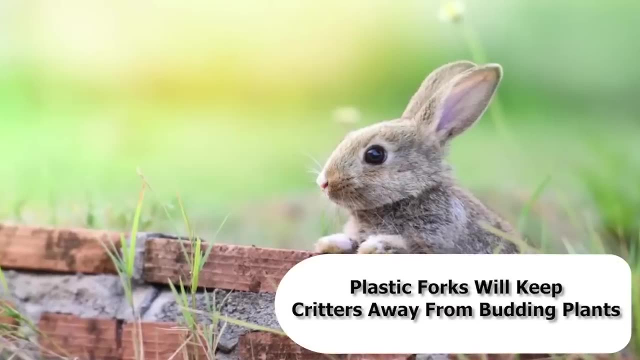 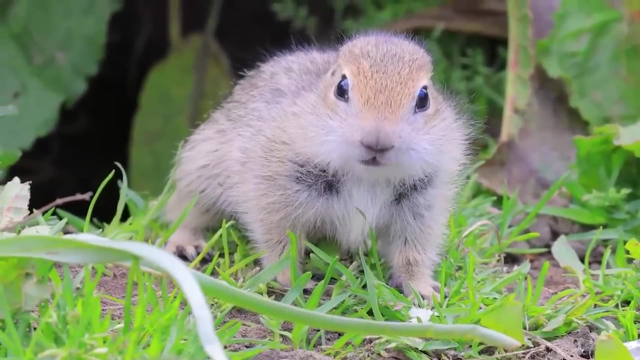 yeast over plants. It's essential to check the level of beer in the can frequently so you can refill it before the can is empty. Keep your focus away from your garden. Plastic forks will keep critters away from budding plants If your dog, cat or outside critters like squirrels and groundhogs get into the garden. 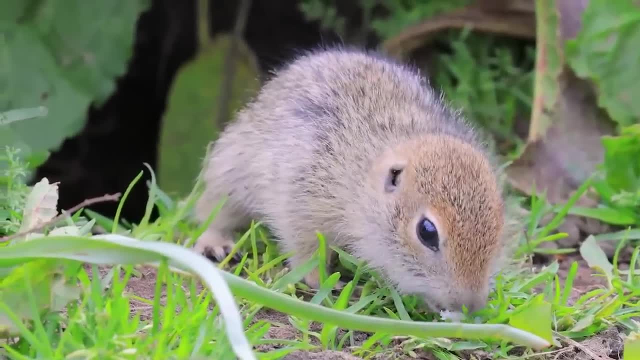 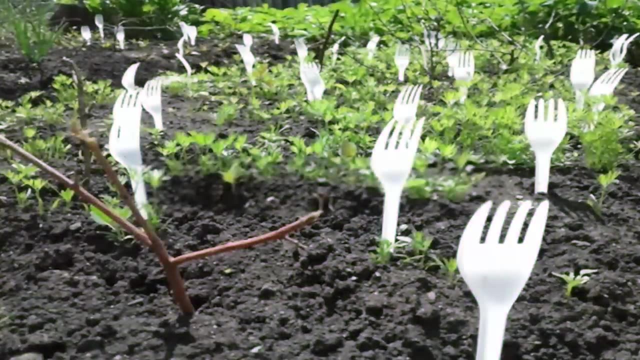 they will eat and destroy the tiny plants that are beginning to grow. Fortunately, there's a simple way to keep animals out of your garden, and all you'll need is plastic forks. All you need to do is push the fork handles into the ground, so only the tines stick out of the ground, and put them. 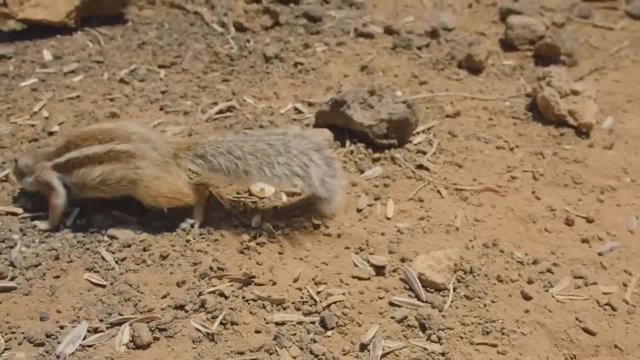 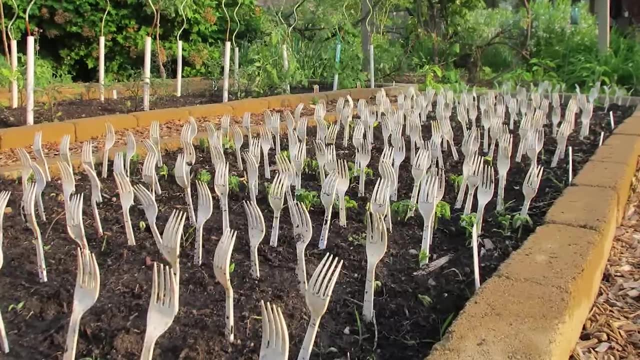 around all of the immature plants. This will deter the animals from walking through the garden, protecting the young plants. The forks can look unsightly, so it's best to use clear plastic forks. You can remove them when the plants have grown enough to stand on their own. 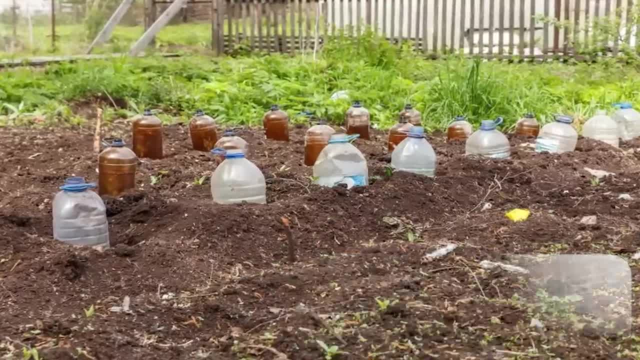 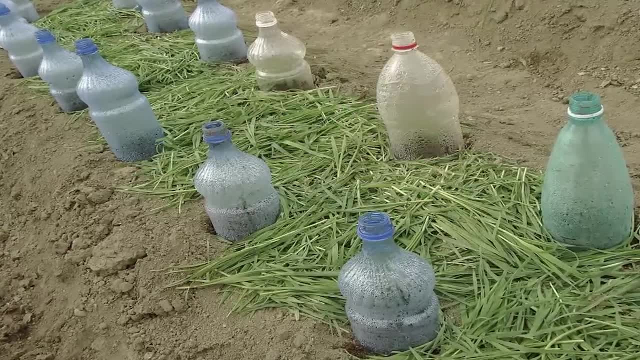 Protect your plants from an early frost. Nothing is worse than seeing a frost warning in the forecast after you've planted the garden. Fortunately, you can protect your plants overnight, as long as you have an empty water or milk jug. Start by cutting the body off. 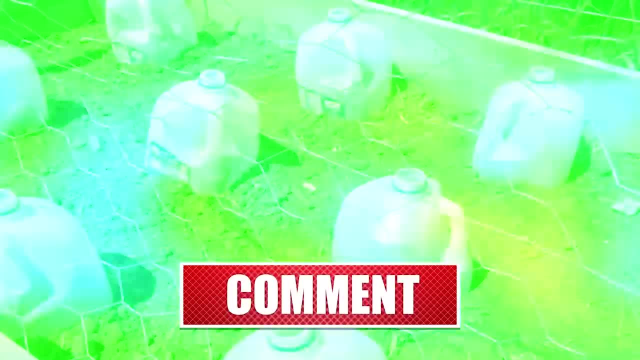 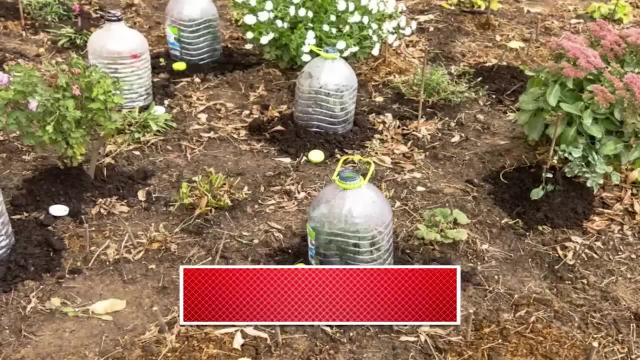 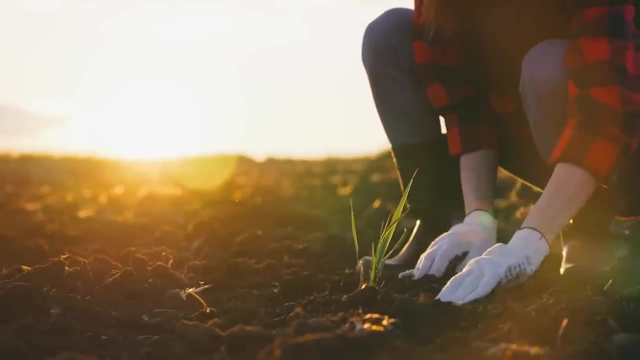 of the jugs and remove the caps for ventilation. Next, bury the jugs in the soil around the plants that need to be protected. This will keep your plants several degrees warmer early in the season, when it still gets cold at night. You can remove the jugs when it gets warmer and your plants are no longer at. 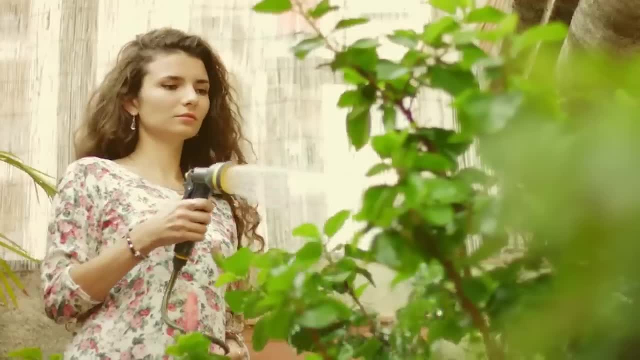 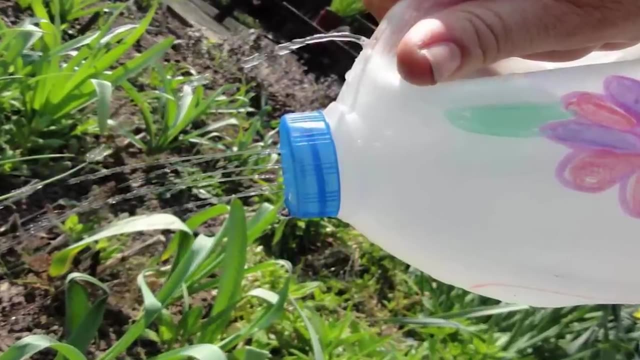 risk. Make your own watering can. If you don't have a watering can for your indoor plants and seedlings, or if your watering can pours too much water, you can make your own using an empty milk or water jug If you're using an empty milk. 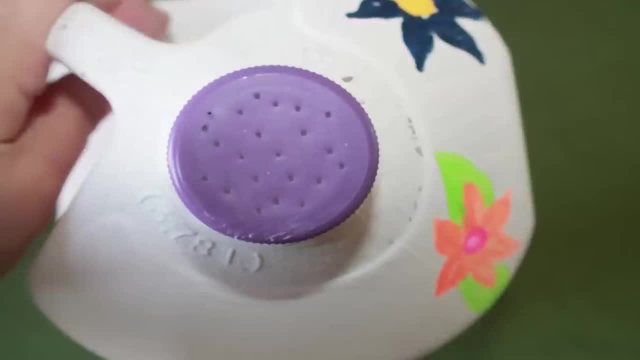 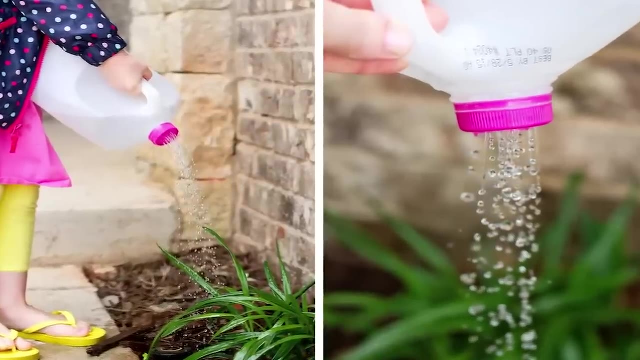 jug, make sure to rinse it thoroughly first. Next, heat a needle to poke holes in the cap. You should poke as many holes as necessary to create adequate water flow. Finally, fill the jug and replace the cover, and you'll have a makeshift. 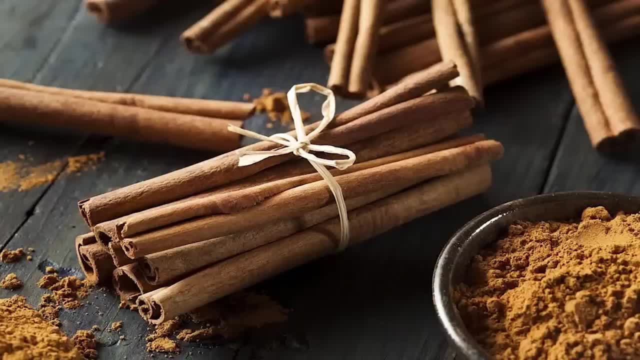 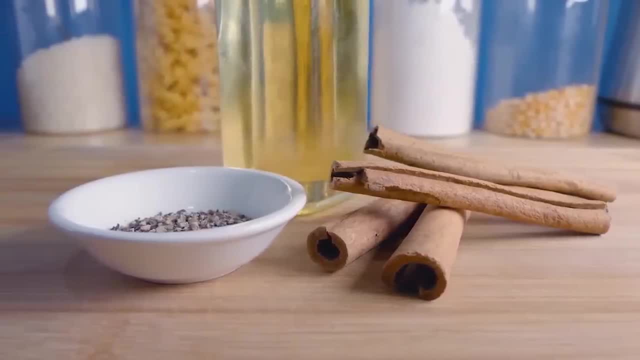 watering can that won't leak and dribble down the spout. Protect your garden with cinnamon. You likely have cinnamon in your spice rack for baking and it can obviously help with the water flow. If you're using a water jug, make sure to. 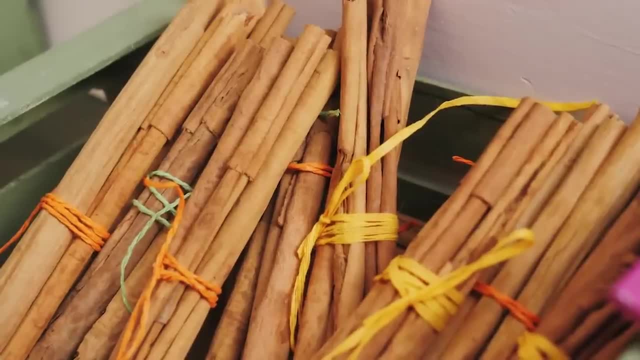 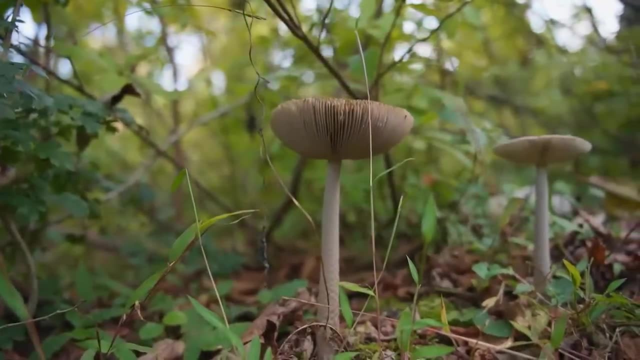 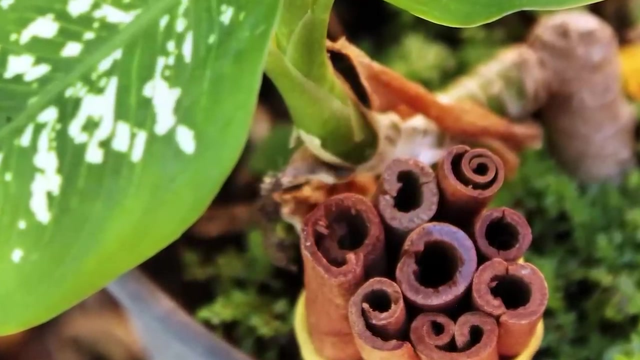 also be used to protect your garden. Cinnamon has antifungal properties that can save seedlings that suffer dampening of disease, and it can also ward off mushrooms and slime mold that can infest your planters. You can also use cinnamon as a rooting agent if you apply it to the stem, and it will also keep the ants. 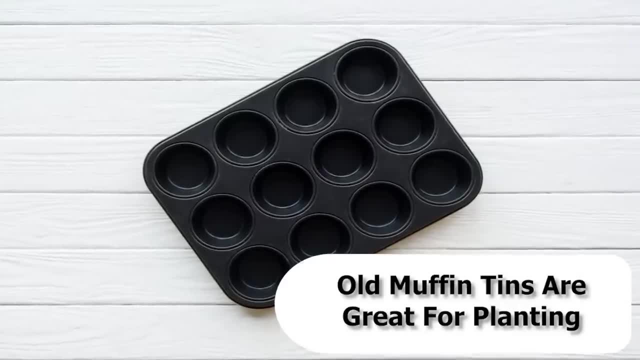 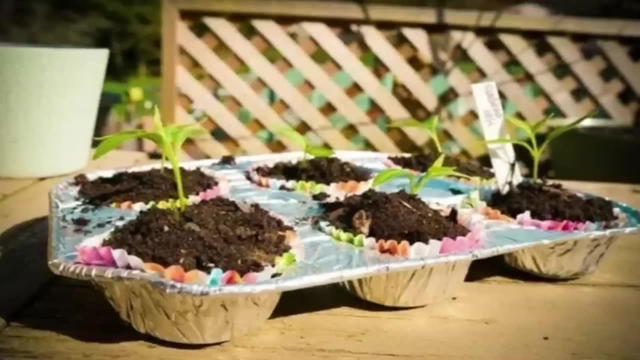 away. Old muffin tins are great for planning. You can put your old muffin tins to use in your garden and they can be used in a couple of ways. First, you can use the muffin tins to start your seedings, and they're the perfect size. You can also use 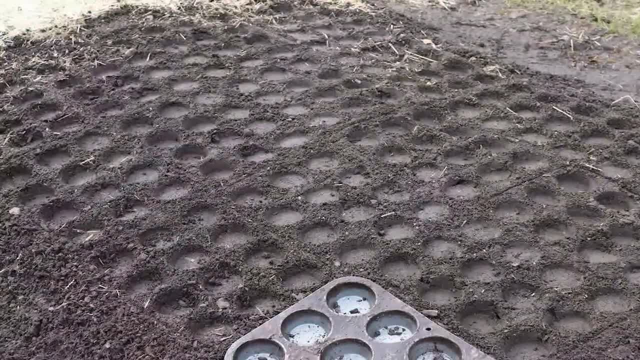 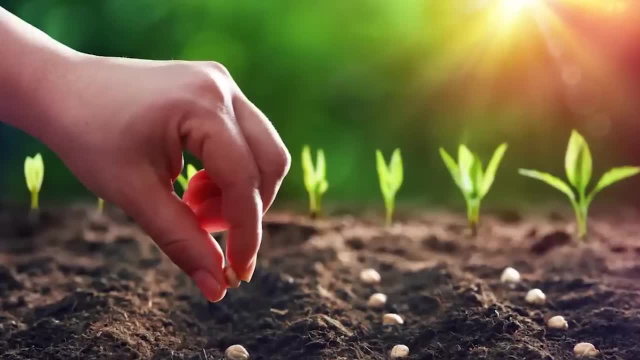 your old muffin pans to plant the garden. When you push the bottom of the pan into the soft soil, you'll have perfectly spaced wells to plant your seeds or plants. When you create the plant grid, dig the holes as deep as you need to plant the seeds and plants. Finally, ensure you don't. 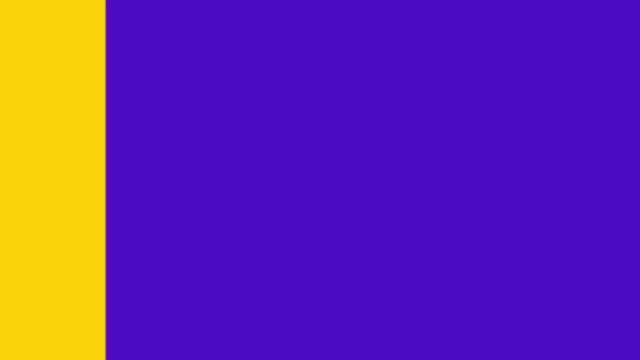 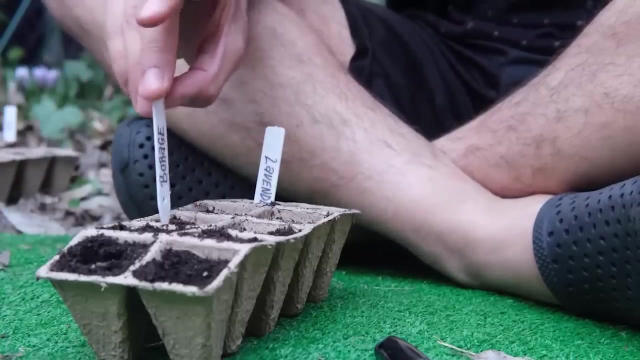 use the tins for cooking because it's incredibly unsanitary. Use old spoons to brighten up your garden. Labeling your plants is a great way to start your seeding. You can also use the muffin tins to start plants. when they first go into the ground is essential so you don't forget what's planted where. 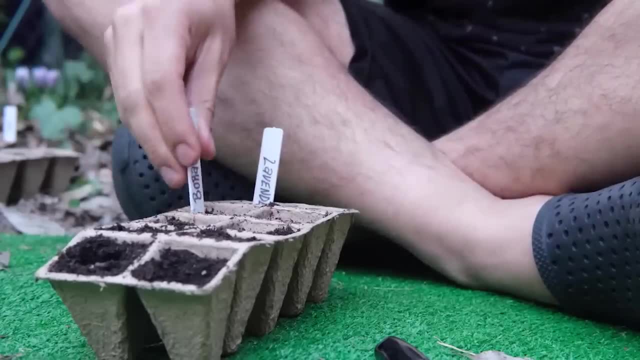 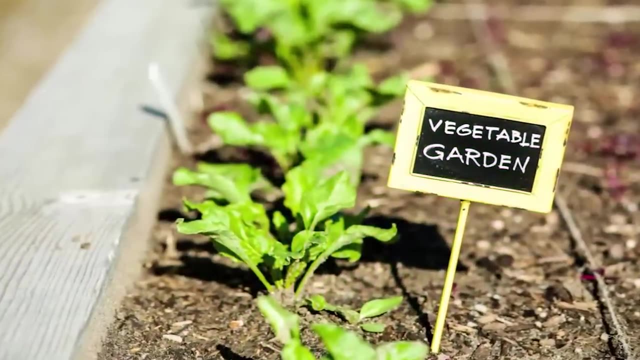 Cardboard garden labels look dull and if you have a bunch of old spoons you can make your own colorful garden labels. Start by flattening the head of the spoon with a hammer, Paint them with craft paint in any design you like and write the names of the herbs and vegetables you have in. 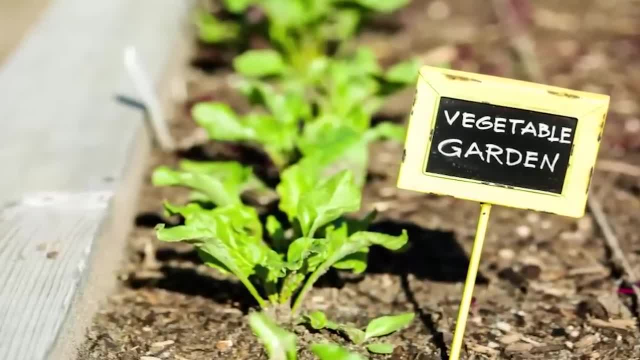 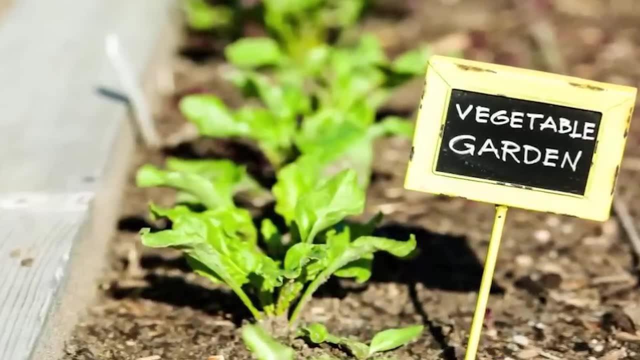 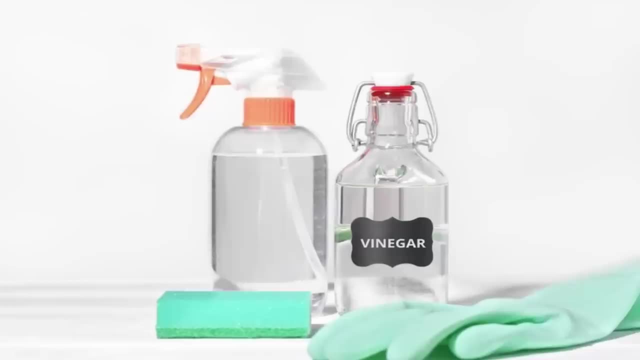 your garden. Finally, stick the spoon handles into the ground so only the label sticks out and faces up. This will brighten your garden and you'll always know where each plant is. Use white vinegar as a weed killer. White vinegar is a natural weed killer and doesn't contain harmful pesticides that you'll find in. 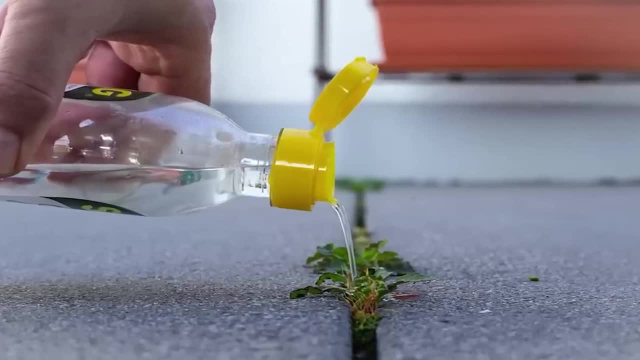 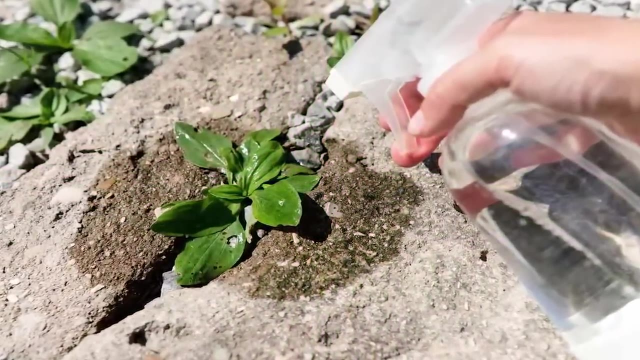 store-bought weed killers. You can spray the vinegar on the weeds, draining the moisture from the leaves and causing them to die. It's best to use this method on a sunny day, because that's when it's the most effective. It's essential that you're careful when spraying the weeds. 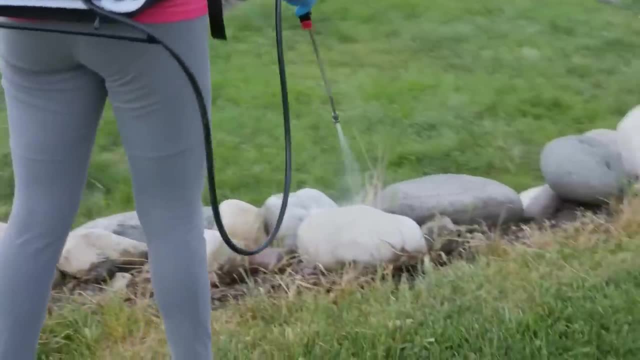 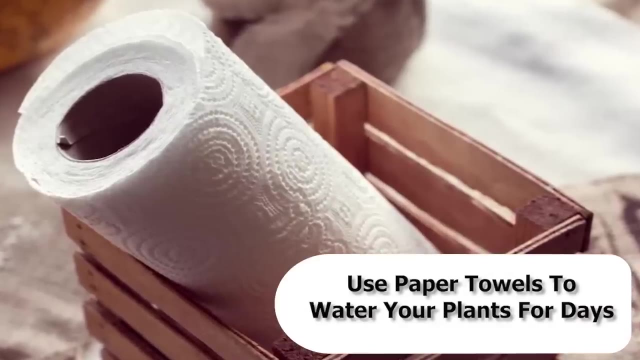 because if it gets on your plants, they will die. Keep the vinegar away from your plants when you spray the weeds and your garden will thrive. Use paper towels to water your plants for days If you're going on vacation and can't find anyone to go to your house and water your plants. 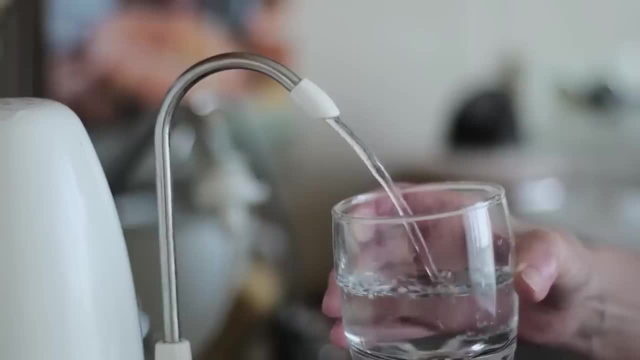 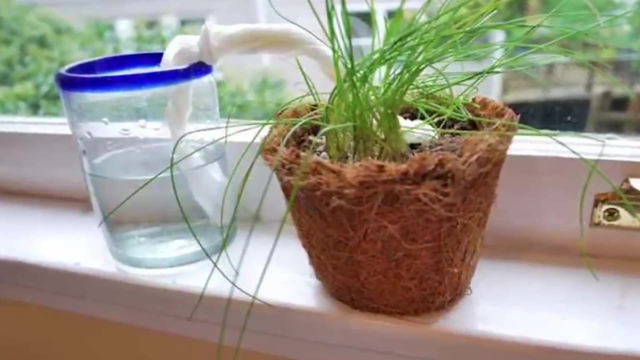 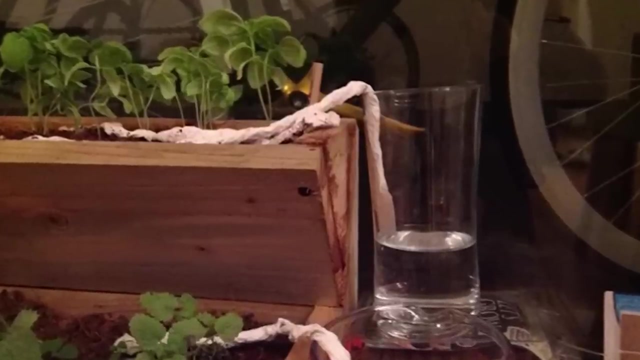 all you need is a roll of paper towels. Start by filling a glass of water and pull about five sheets of paper towel off the roll. Next, dampen the paper towel and spread one end evenly over the soil. Put the other end all the way down in a full glass of water. so the 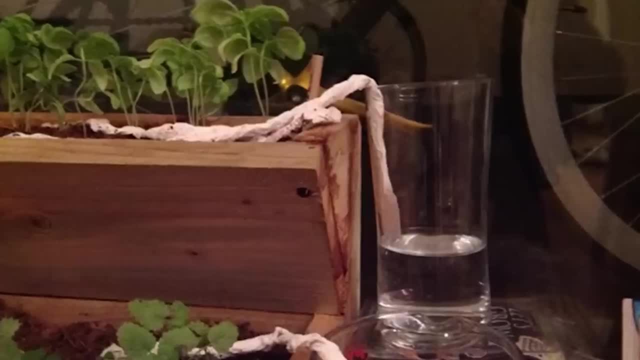 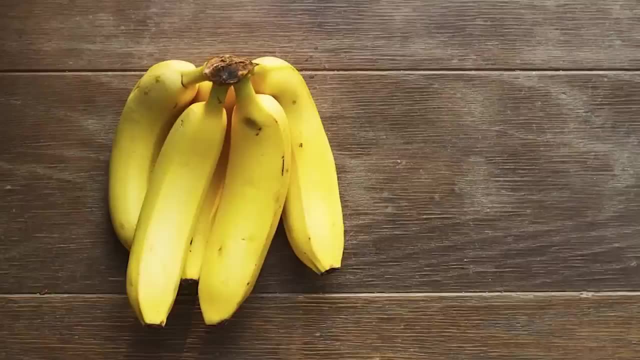 towel remains moist and you won't have to worry about watering your plants until you get home. This hack is much cheaper than hiring a house sitter to water your plants. Bananas Will Help Your Garden Thrive. Plant bananas in your garden. Here's what. 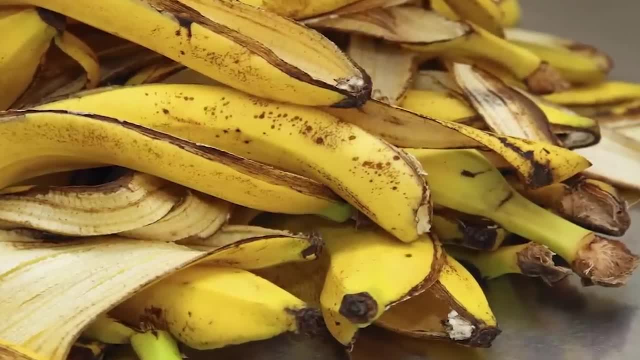 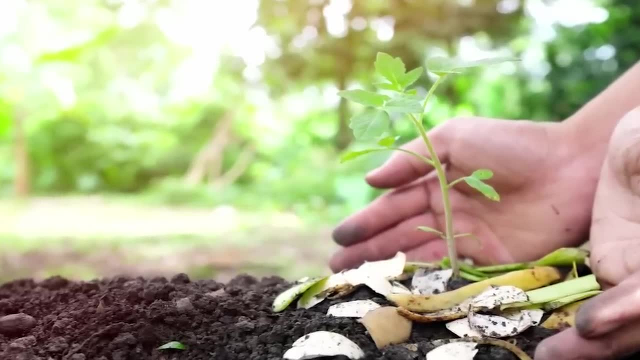 happens, You don't have to plant the whole banana in the garden and you should only use the peel. Banana peels are a great addition to the soil because they are rich in sulfur, magnesium, calcium, sodium, phosphate and potassium and can help your plants flourish. 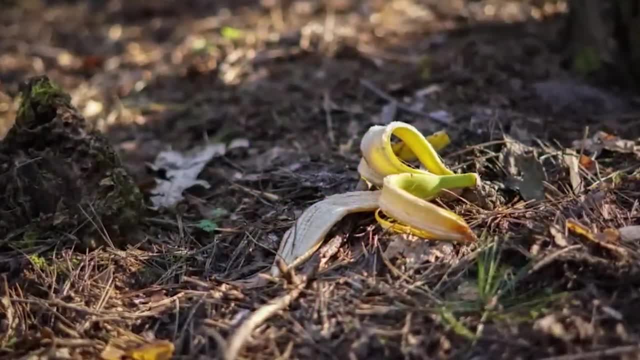 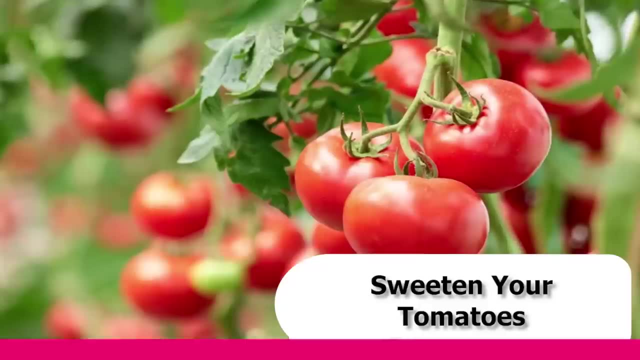 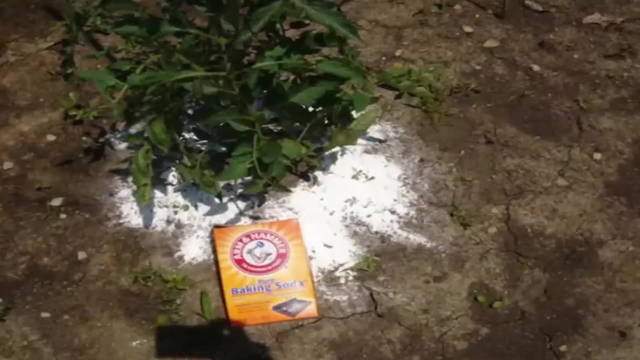 Banana peels break down quickly and the nutrients will absorb quickly. Cut up the peels and mix them in the soil and compost, and your plants will thrive. Sweeten Your Tomatoes If you prefer sweet tomatoes. you can achieve this goal using baking soda. Surround the base of the tomato plants with. 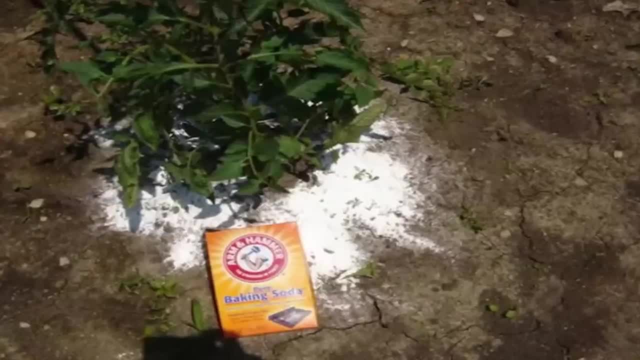 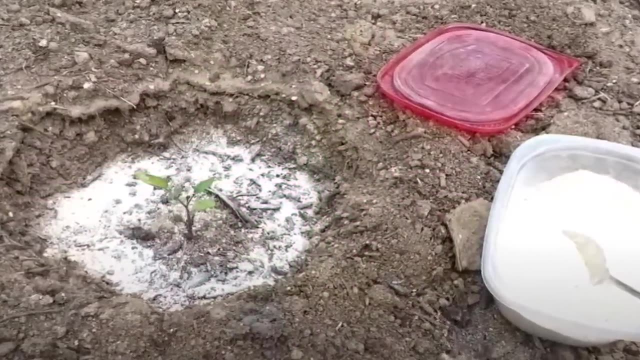 baking soda and the plant will absorb it through the roots and this will sweeten the soil. The baking soda can kill the plant's leaves, so make sure you only put it around the base of the plant. Make a Planter with an Old Colander. 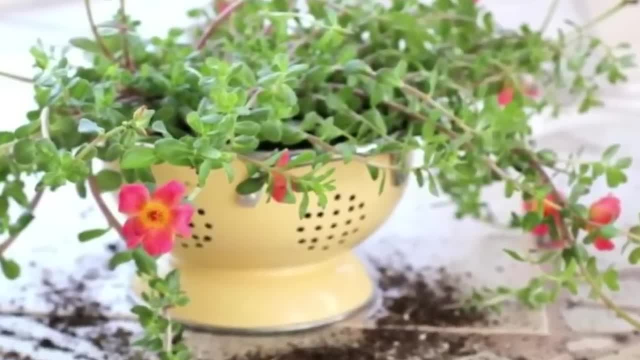 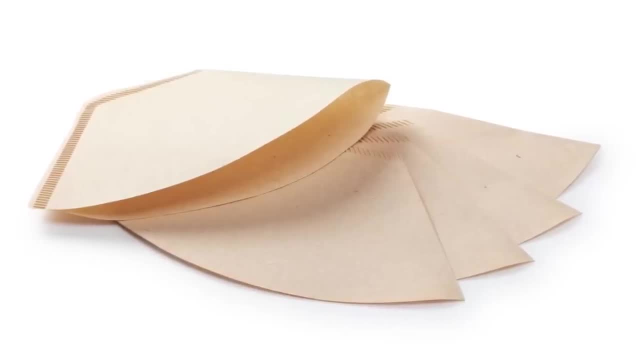 If you don't have any planters and have an old colander or strainer you didn't have the heart to throw away, you can use it as a planter. Start by lining the bottom of the colander with a coffee filter and then add the soil and the plant. The filter will keep the soil. 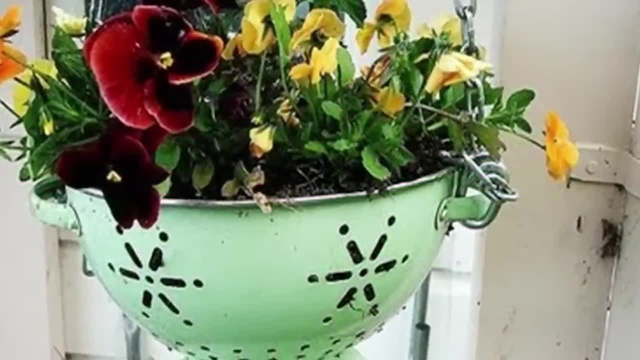 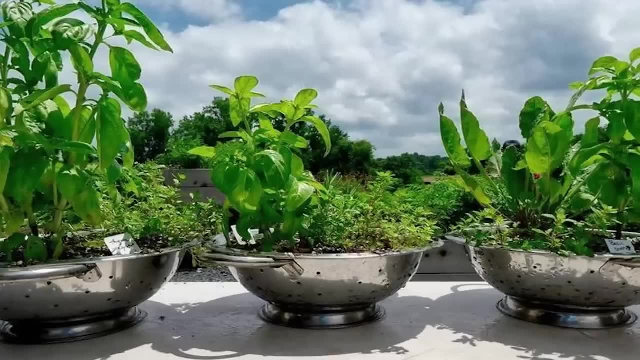 from falling out of the holes and the water will still drain. You can add a sturdy rope or chain to make a floating planter. Start by lining the bottom of the colander with a coffee filter. Create Your Own Mini Greenhouse. Greenhouses help plants thrive because 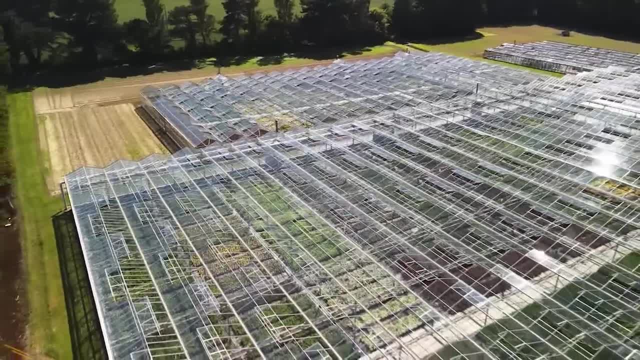 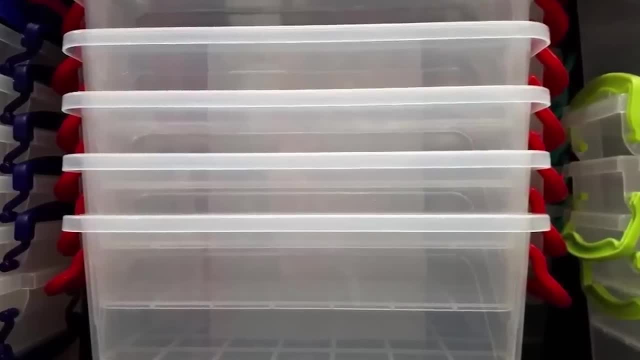 they let the light in and don't let the heat escape. Greenhouses are very expensive to build, but you can make your own for a fraction of the cost using clear plastic storage bins. All you need to do is take the potted seedlings you would typically put in the window and put them.